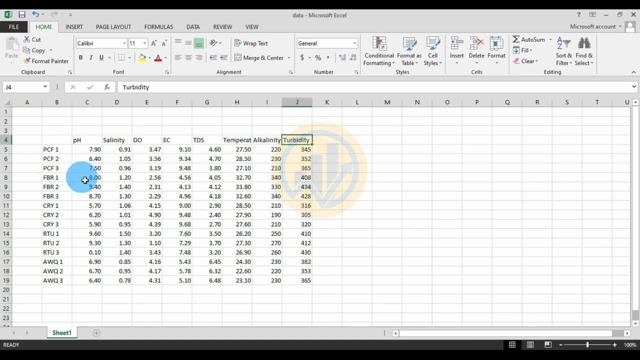 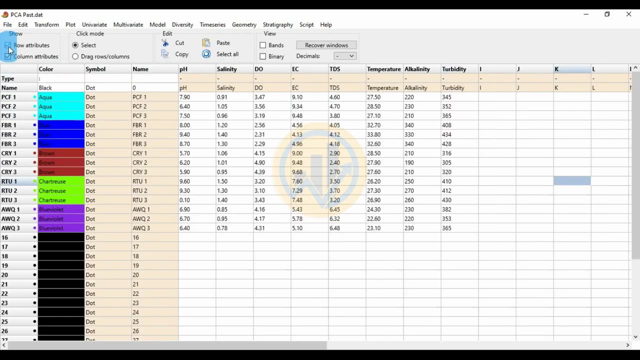 temperature, alkalinity and turbidity. This data copy paste to the past statistical software. The data copy Copy Then go to the past statistical software The data already entered. So first click the column attributed, Then row attributed, Select the zero column, Then paste the data, Then color change for 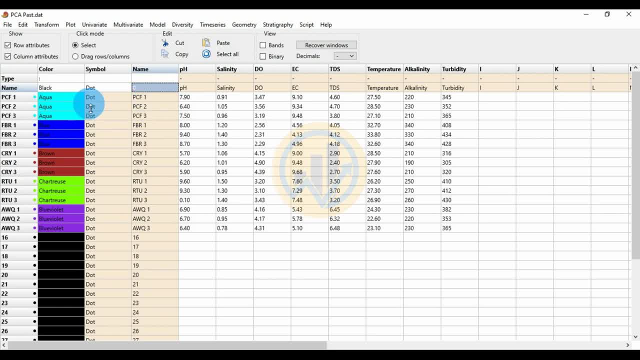 the group For the PCF, 1,, 2, 3, the same color. and the FRB, 1,, 2, 3, the next one color. The third one for the CRY, 1,, 2, 3 is a different color. Then next one shows color for the RTU. 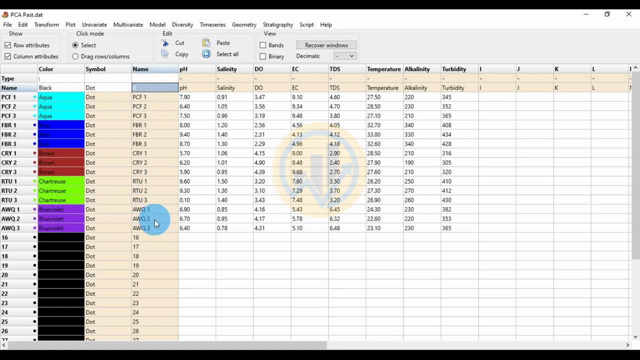 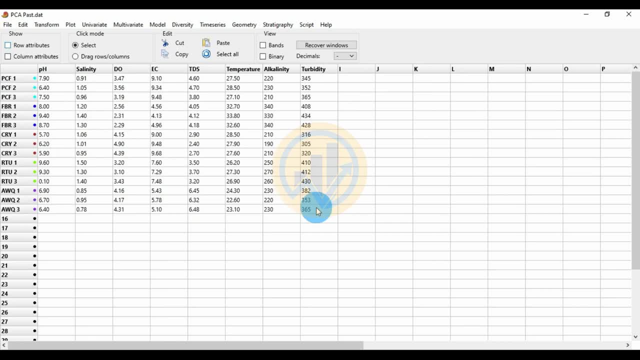 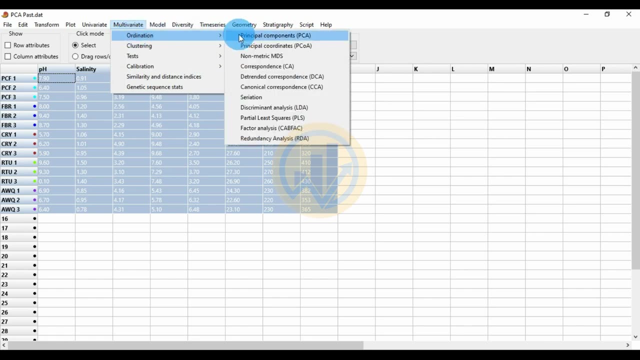 1 and 2 the same color, Then AWQ 1, 2, 3 the different color, Then unclick for Russian column attribpper and ROH attribpper. Then select the data, Go to the multivariate menu, Click the ordination and click the principle computer analysis. 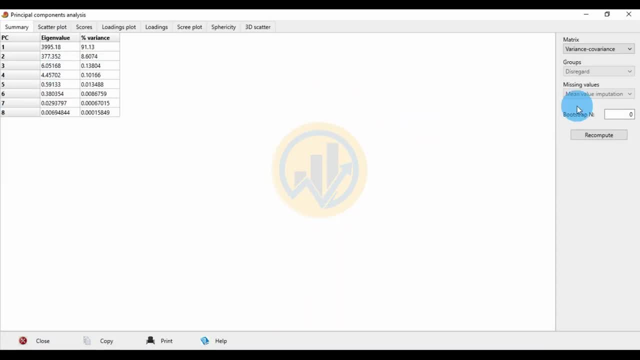 This is the principal component analysis For the matrix value. click the correlation and then click theронut machine button. Click the recompute button. The equ cable value for the 4 points is highest value in the 4.28931 tease and the variation. 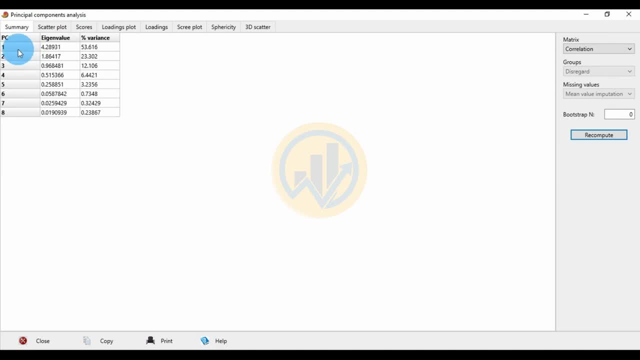 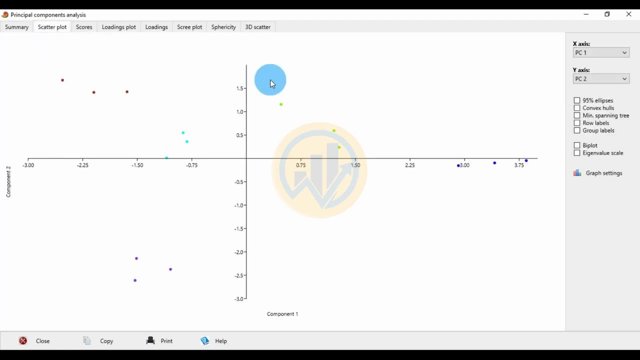 percentage in the highest percentage value for the principal compound analysis. one fifty three point six. one six. the next one for the scatter plot for the principal compound analysis graph. just to the graph for the click the biplot checkbox, the try a elemental water parameter, the temperature, salinity, alkalinity, terminity, pH, DDS, DO and EC, and the next one row label, the. 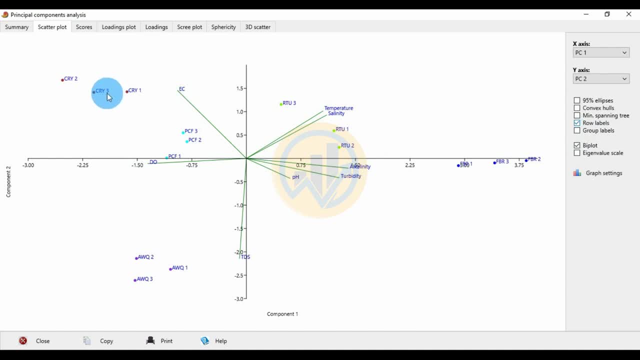 click the checkbox, the row label for the water sample parameter, then action for the principal compound analysis. one: this is a principal common analysis. one, then next one for the principal common analysis to the principal common analysis. two, for the y-axis, the principal component analysis. one is a XHS, the change for the principal common analysis. one, two, three, four, five, six. first one: 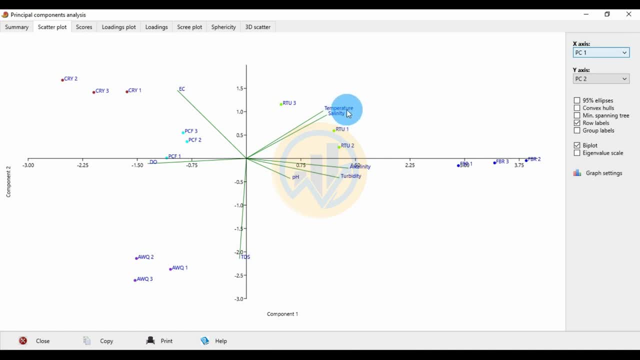 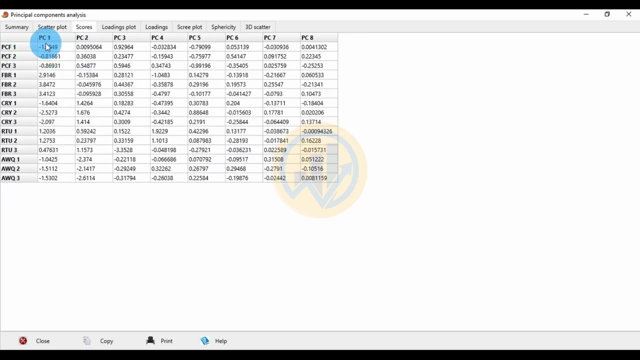 for the as a correlation for the positively presented in temperature, salinity and EC, The negative correlated for the alkalinity terminity, pH, DDS and DO, The score value for the scatterplot, the first one for the PCF 1,, 2,, 3.. The principal: 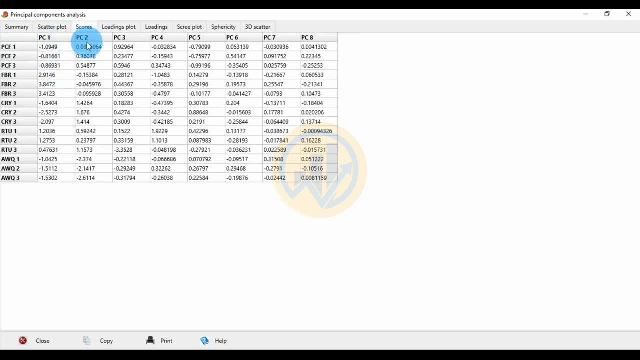 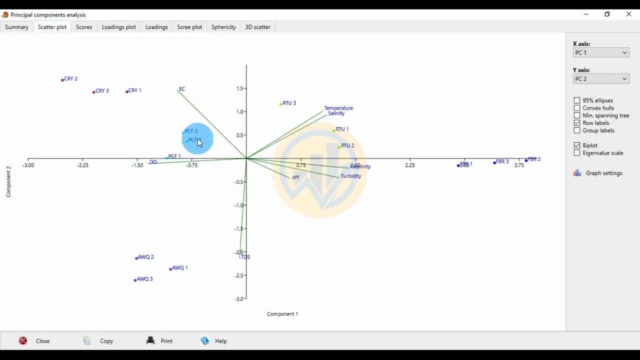 component analysis on the negative correlated and principal component analysis to the positive correlated PCF 1,, 2, 3. The PCF 1, 2 and the negatively correlated for the DO and positively correlated for the EC, the principal component analysis. 2. The next one value for the FBR, The 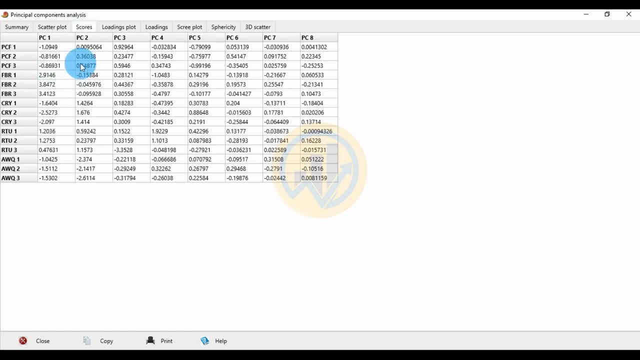 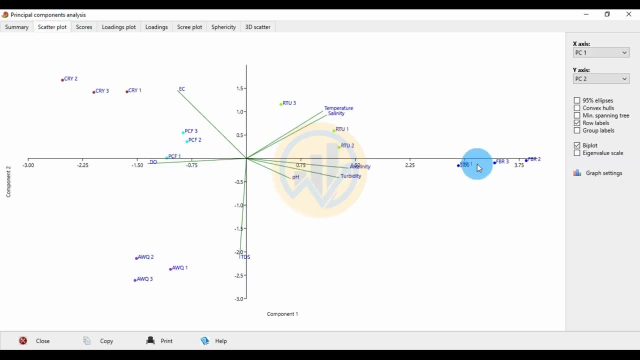 FBR. the first principal component analysis is positive. The next principal component analysis, 2, is a negative correlated FBR. The FBR value present, the first one for the positively correlated in the terminity and salinity, Then negatively correlated for the alkalinity, terminity and pH. 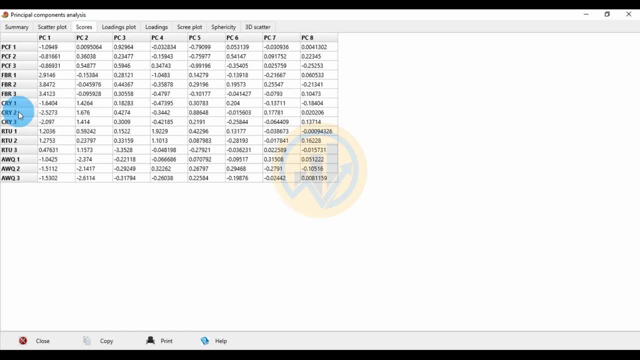 Then third, one for the CRY1,, 2, and 3.. The negatively correlated in the principal component analysis: 1 and the principal component analysis: 2.. The positively correlated, The same. also the three: the PC1, the negative, and the PC3 for the positive, The PC4 for the negative, PC5 is a positive and the PC6 is a negative, And 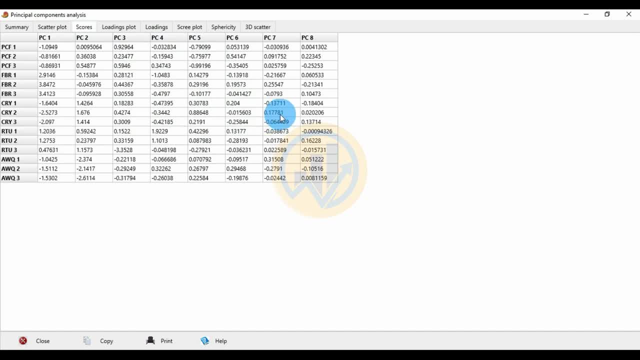 the PC7 for the CRY, the positive, The PC8 for the positive in the CRY, Then next one for the RTU1, 3.. The principal component, one, the positive, and the second, also the positive, The RTU. 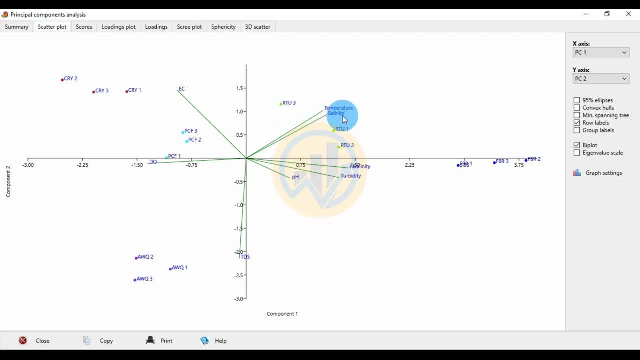 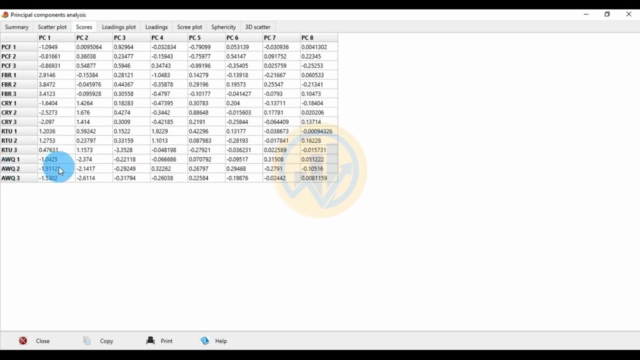 the first, the positive for the correlation temperature and salinity. That also the EC also said is the positive correlated it. The next one for the 2 value, the principal compound analysis 2 and 1.. also the negatively correlated for the AWQ: 1, 2. 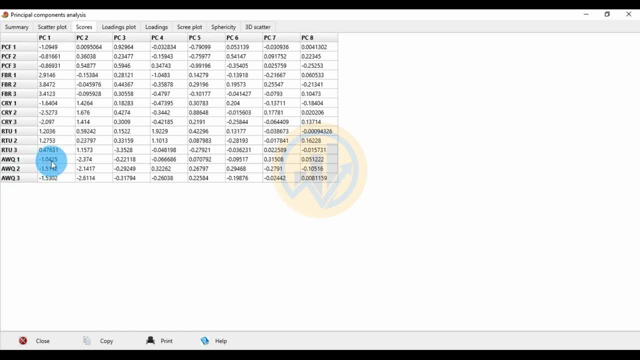 or 3.. The third one, negative value for the negative, for minus 1.0425. The AWQ, the negatively correlated first value for theかった view is 3.. The negative value for minus 1.0425.. Thespetr, first one for the negative: 15, is negative. 16, will be the first value given. Next one is the every 7,, 7 and galactic rate. 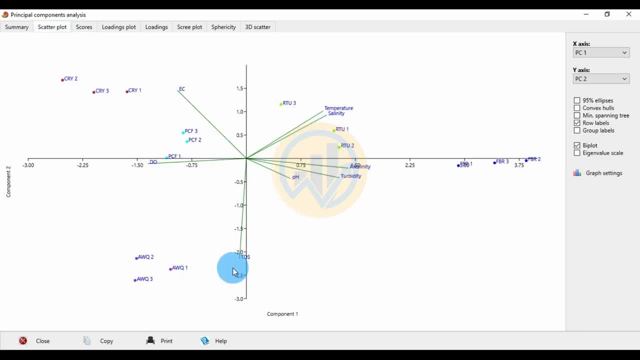 For the每 2, 3wh. 저는 gyn厍 nêo gêbl developments. 2. edge point scale: The AWQ, the negatively correlated first value for the score value. principal component analysis: 1, the 1.04.. 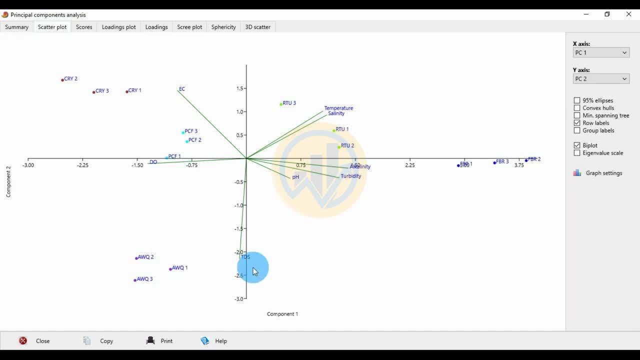 The A point for the 1.04.. The next is the 2 point for the minus 2.374.. Minus 2.374 for the principal component analysis: 2.. This is a principal component analysis. 1.. This is a principal component analysis. 2.. 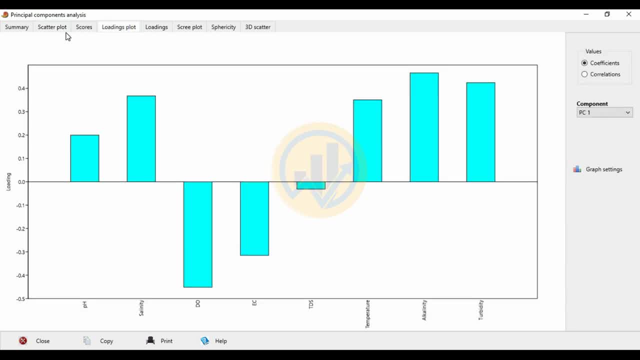 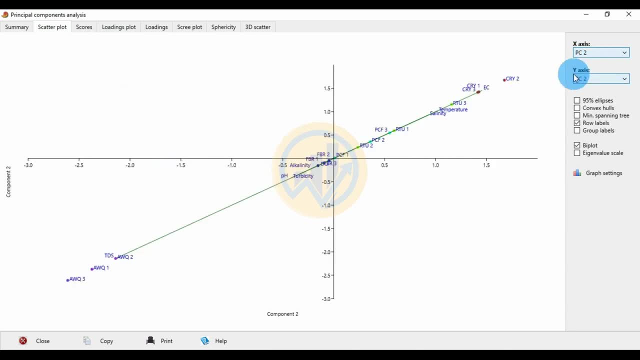 The next one for the loaded scatterplot. Before we check the scatterplot: change for the XHS: principal component analysis 1, the comparison for the 2, the XHS, also same PC2, PC to the scatterplot. Then next one for the change: the XHS value, the PC3, principal component analysis 3 and principal component analysis 4 and the principal component analysis 5.. 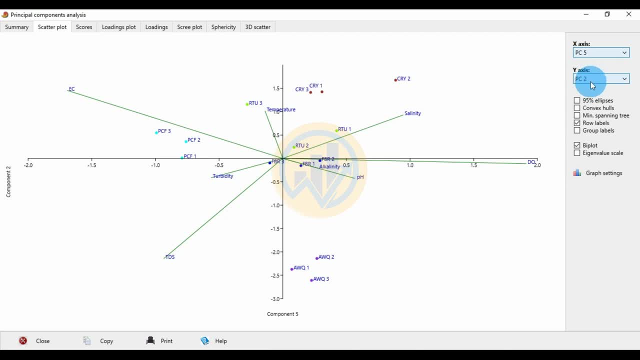 The principal component analysis 5, XHS and principal component analysis 5.. Y is a: 2. Then value for the first one for the RTU 1,, 2, then this chamber, the different chamber, for the RTU 3.. 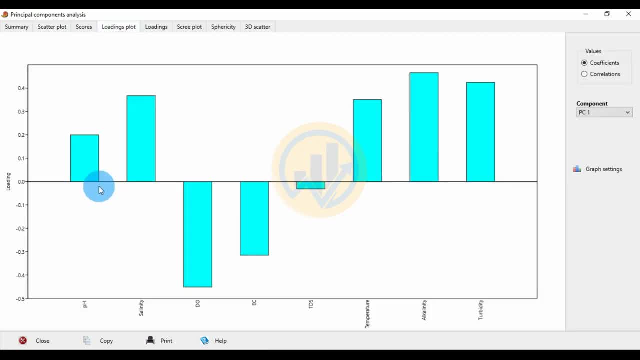 Then next one for the loading plot. The loading plot for the positively correlated PC1, the PC1, click the value for the correlation. the component for the principal component analysis: 1. The positively present: the pH, salinity and temperature, alkalinity and turbidity. 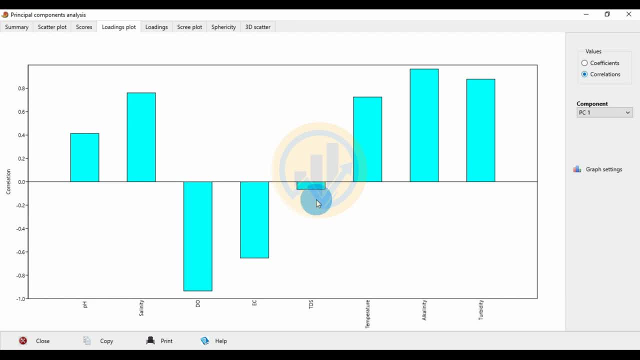 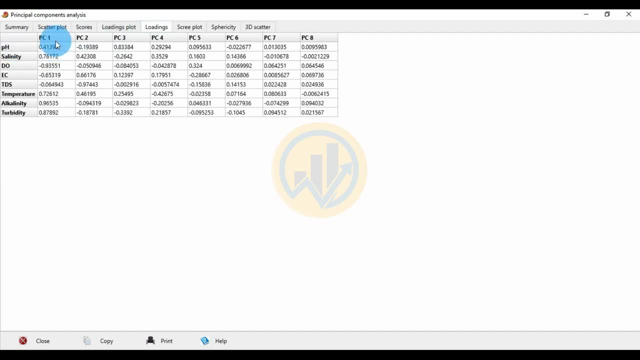 The negatively presented Here in the DO, EC and DDS. The loading plot value for the next slide. The loading plot for the first one for the principal component analysis: pH salinity value 1.01, 0.41.. The pH is 0.41.. 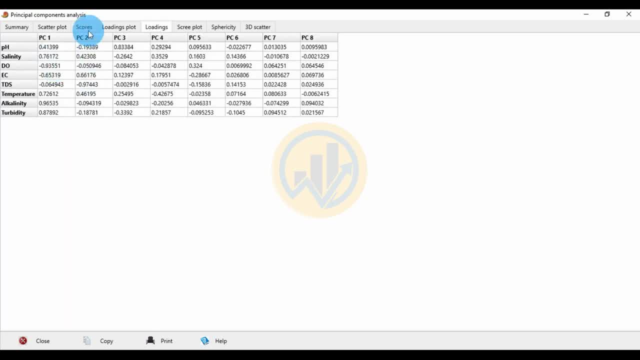 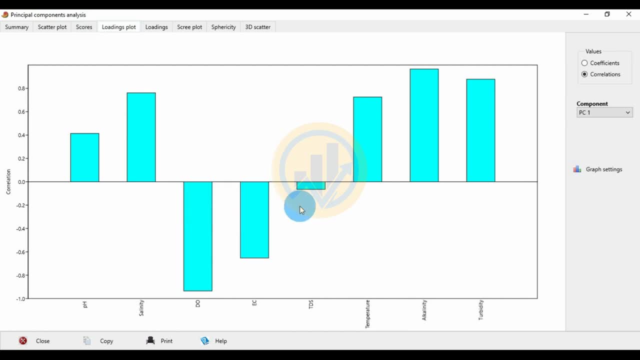 The next one for the salinity: 0.76.. 0.. value for the 76.. The next value for the negatively correlated for the DO, EC And DDS: The negative correlated for DO: the value 0.93.. The EC: 0.65. 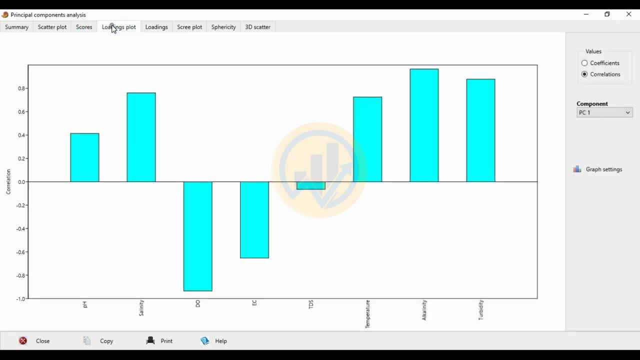 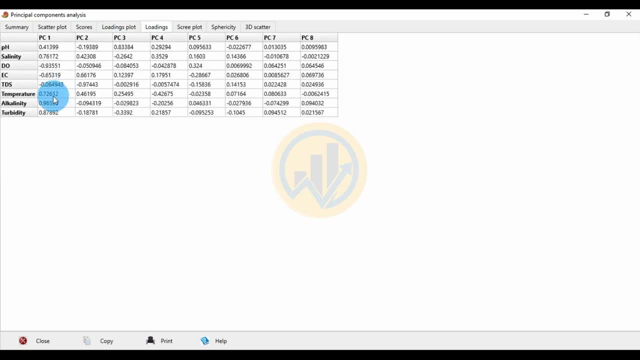 And DDS 0.064.. 0.064.. Then positively correlated for the temperature, alkalinity and turbidity. The positively correlated for the turbidity And the next one for the principal component analysis. 2. The first one for the pH, negative correlated. 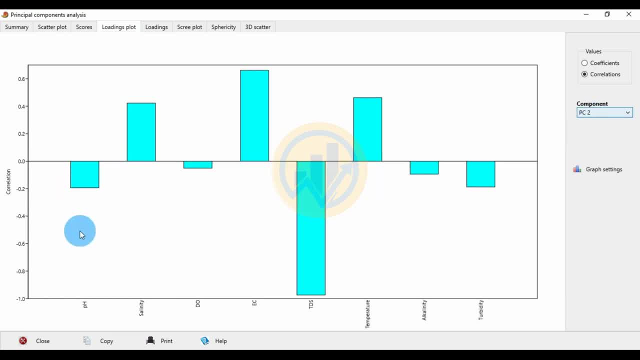 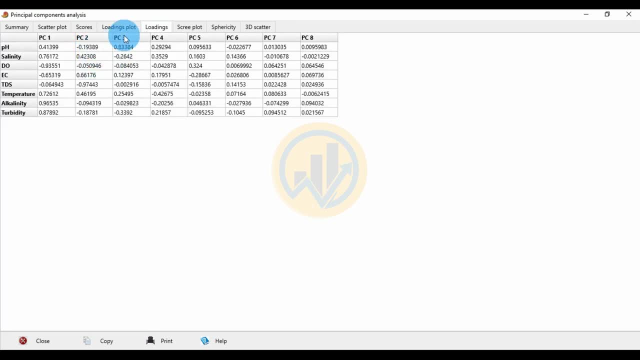 Change for common for principal component analysis. The first one for the pH is negative, The score value for the minus 0.19389.. The next one for the salinity and the EC and the temperature. Also the positive correlation, the PC2.. 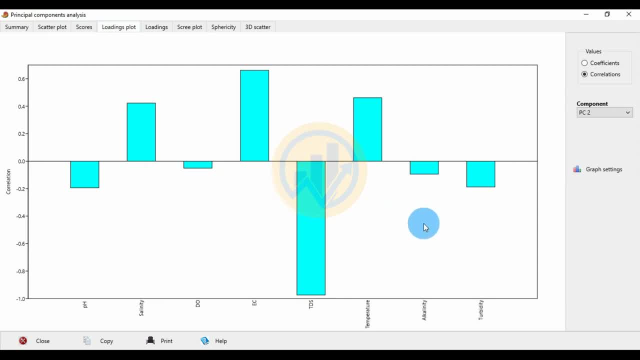 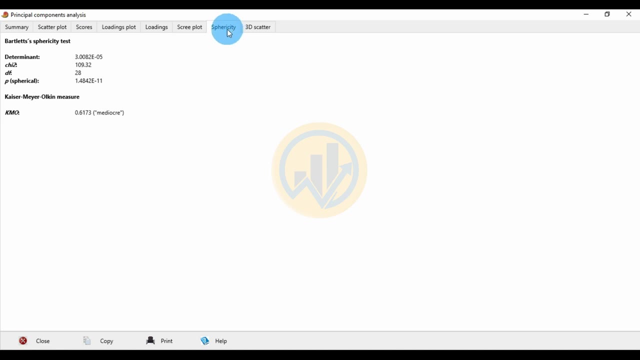 The negatively correlated for the pH, DO, DDS, alkalinity and turbidity is a negative correlated. Next one for the scatter plot. This is a scatter plot. Next one for the test, for the Bortless Peer city test. The Bortless sphere test is test for the determination value. 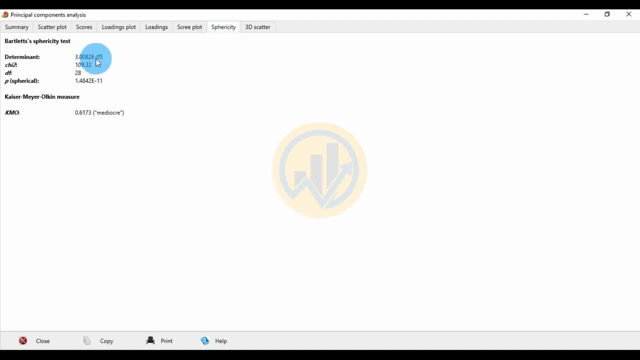 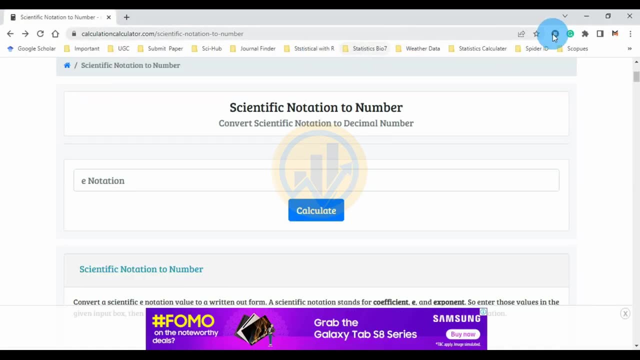 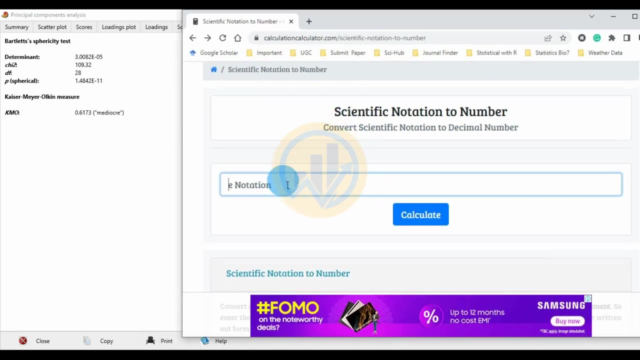 3.0082E to the power minus 0.5.. This is a scientific value Convert for the numeric value. This link is mentioned for the description box Converter: Online converter. Enter the value: Scientific value: 3.0082.. 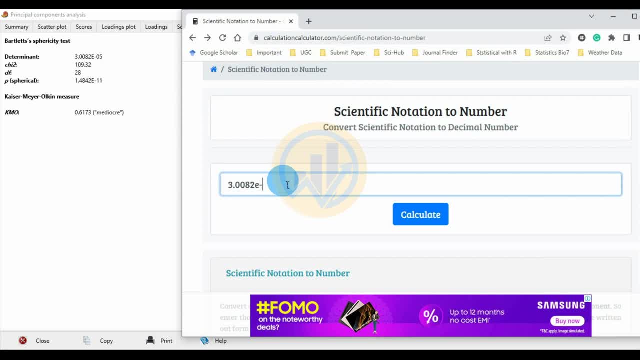 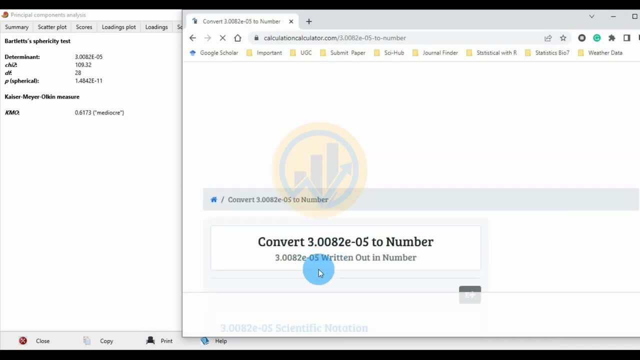 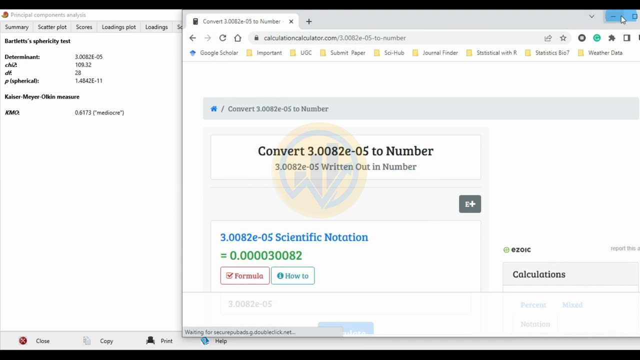 Minus Small e Enter the small e Minus 0.5.. Click the calculator. The determinant value for the 0.4030082.. The next one for the High square test value: 109.32.. 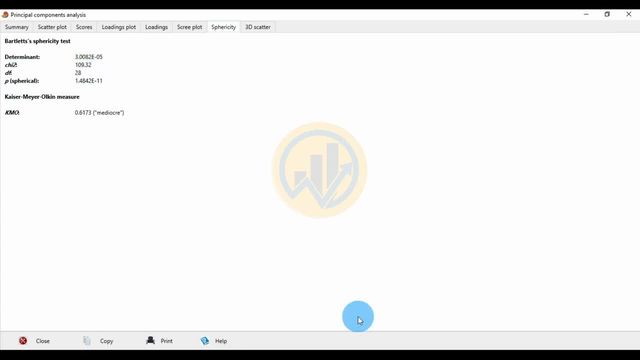 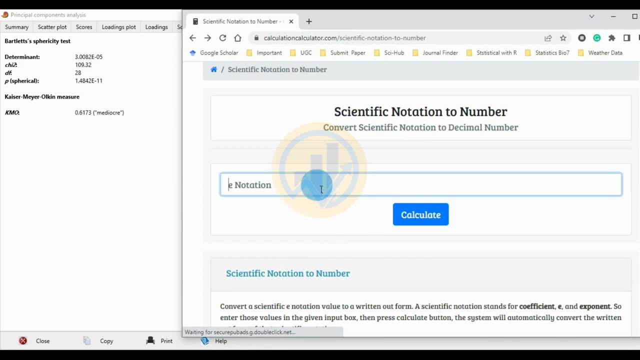 The difference of freedom 28.. The next one, P value. for the P value, Go to the back. Enter the scientific value 1.4842.. Enter the small letter e To the power minus 11.. Click the calculate button. 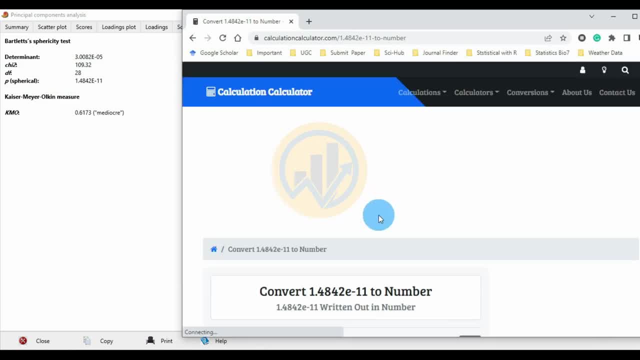 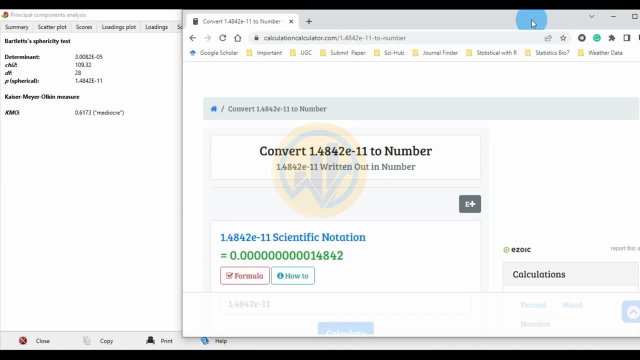 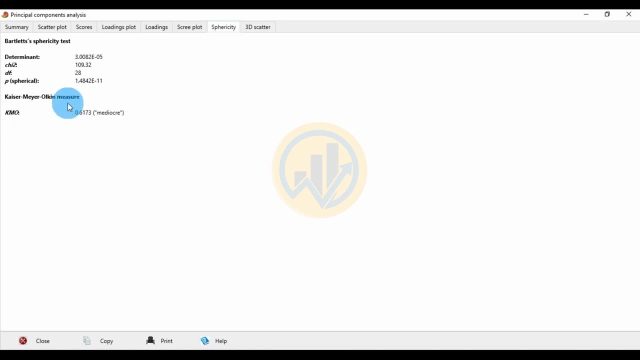 Click the calculate button. The value 0.1014842.. The statistically significant. The next one test for the Higher Meyer: Heiker Meyer test, the measurement, the hulk and mayor walking measurement. then kmo: the measurement value for 0.6173. 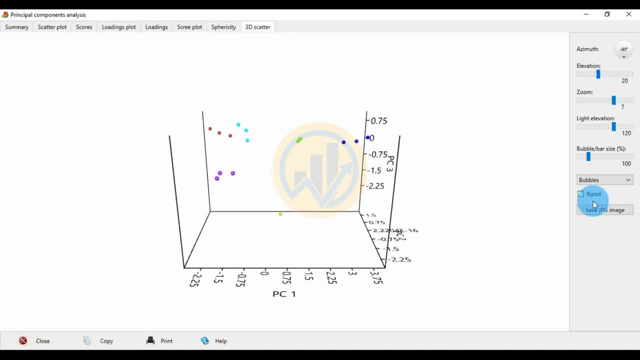 then next one for the 3d scatter plot: the click, the buy plot, the. this is a 3d graph for the scatter plot, the movement graph for the adjustment 90 degree: 40, 20, 30. this is adjustment for the 3d scatter plot in principal compound analysis. 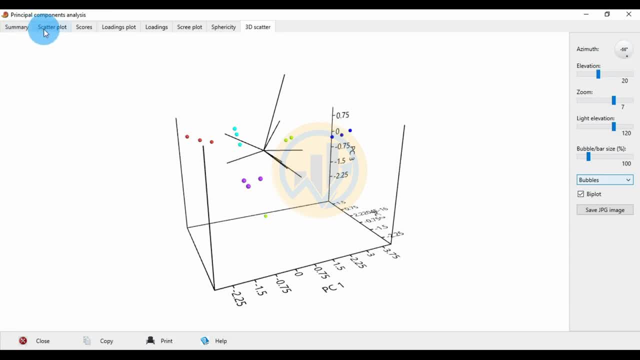 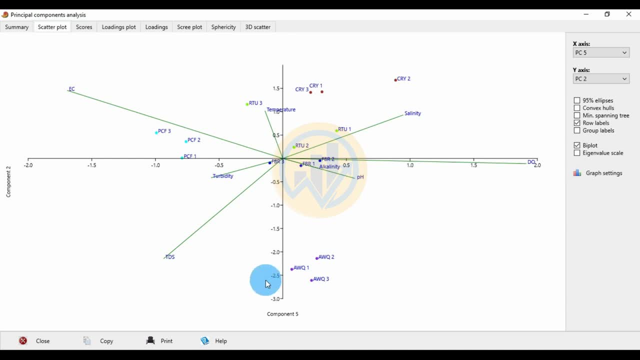 adjustment for the graph in the principal common analysis. thank you for watching this video. if you like our channel, please click the subscribe button. you.